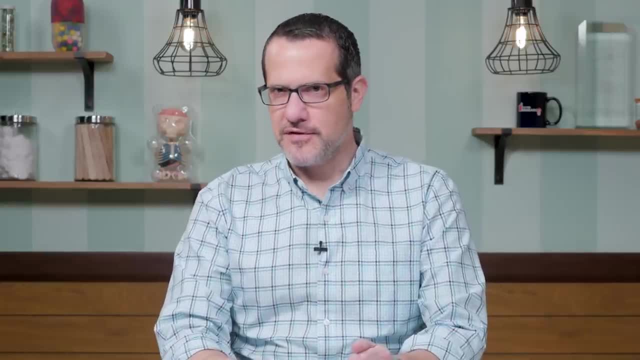 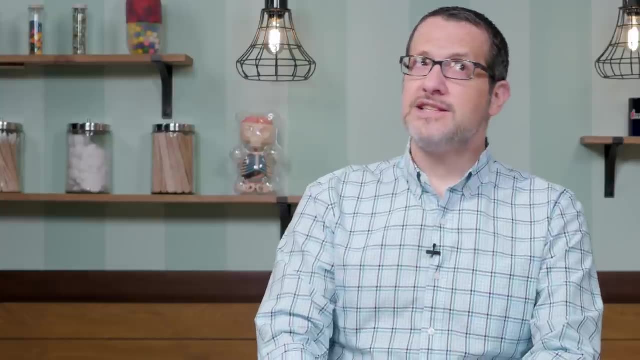 You might think that once drugs, devices and medical procedures are shown to be effective, they quickly become available. You might also think that those shown not to work, as well as alternatives, are immediately discarded. Reasonable assumptions both, but you'd be wrong. That's the. 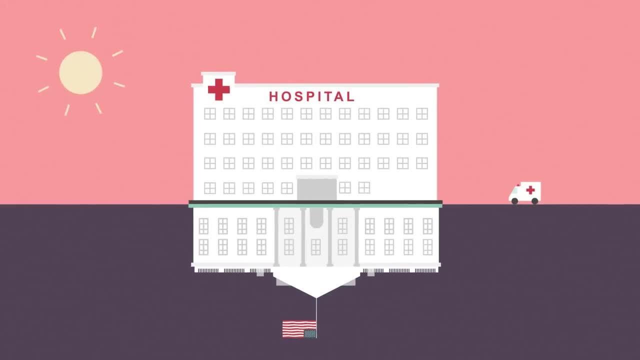 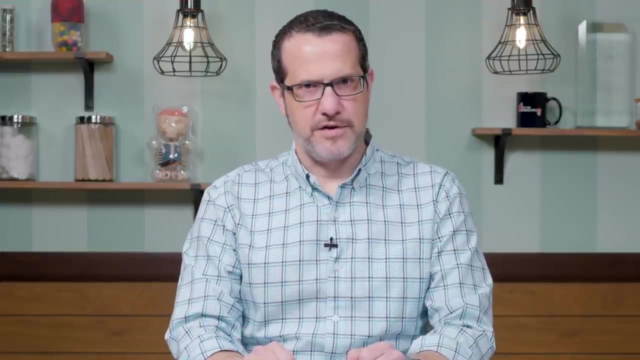 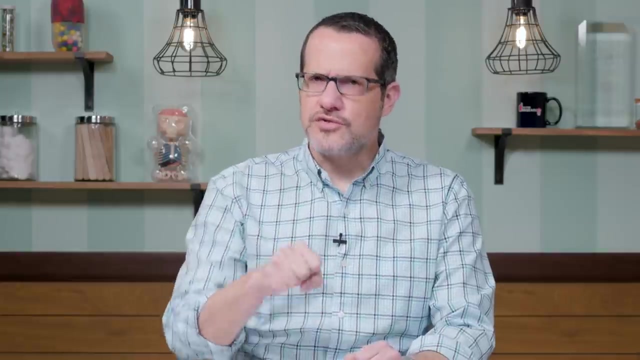 topic of this week's Healthcare Triage. Innovations in healthcare diffuse unevenly across geographic regions, not unlike the spread of a contagious disease, And even when studies show a new technology is overused, retrenchment is very slow and seemingly haphazard. 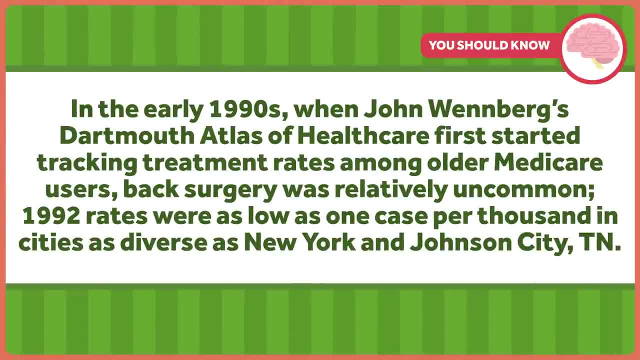 Back surgery is a great example. In the early 1990s, when John Wenberg's Dartmouth Atlas of Healthcare first started tracking treatment rates among older Medicare users, back surgery was relatively uncommon. 1992 rates were as low as one case per thousand in cities as diverse as New York. 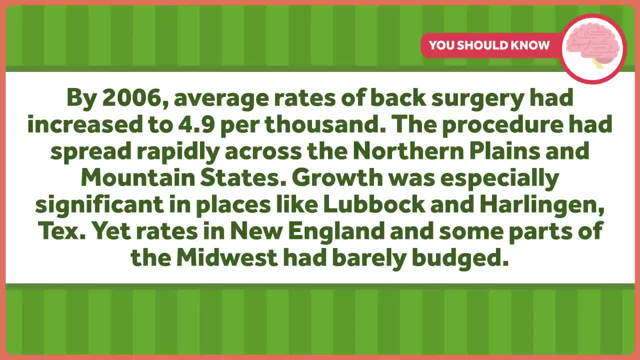 and Johnson City, Tennessee. By 2006,, average rates of back surgery had increased to 4.9 per thousand. the procedure had spread rapidly across the northern plains and the mountain states. Growth was especially significant in places like Lubbock and Harlingen, Texas. 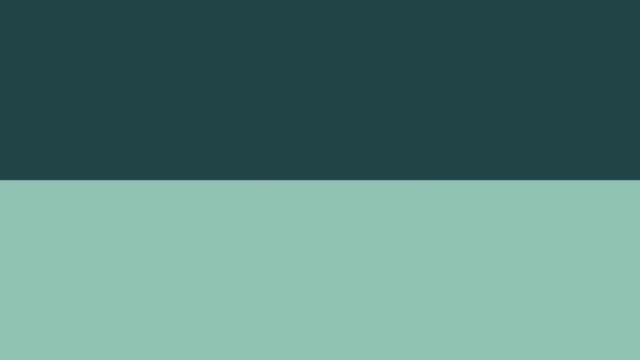 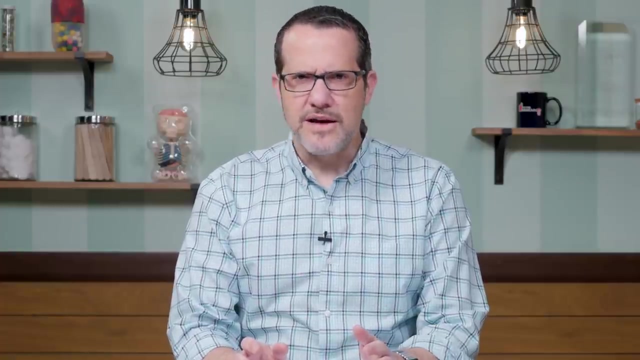 yet rates in New England and some parts of the Midwest had barely budged. Even as back surgery's popularity as a treatment for back pain began to rise in the 1990s, there was little solid evidence of its effectiveness. It wasn't until 2006 that 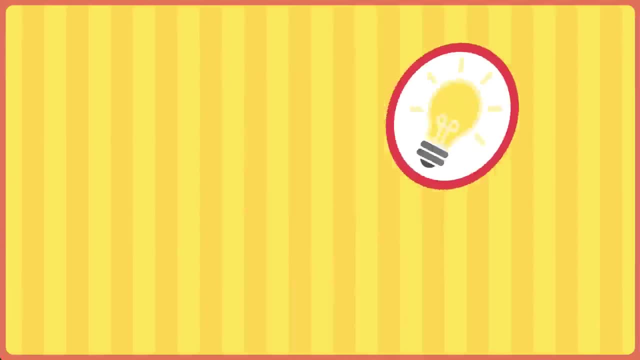 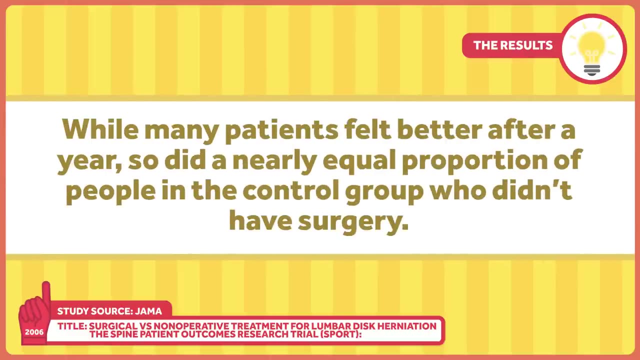 the first large randomized controlled trial on the subject was published. That study showed relatively modest benefits of surgery for many conditions that led to back pain. While many patients felt better after a year, so did nearly an equal proportion of people in the control group who didn't have surgery. 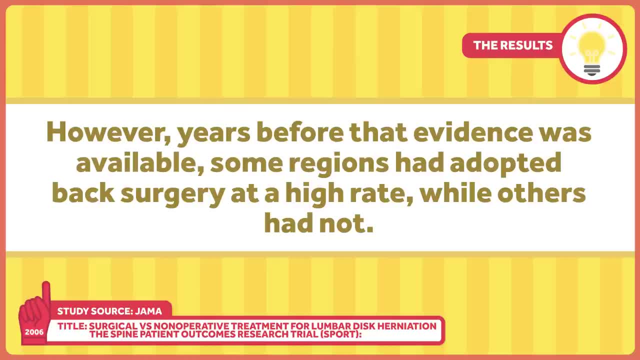 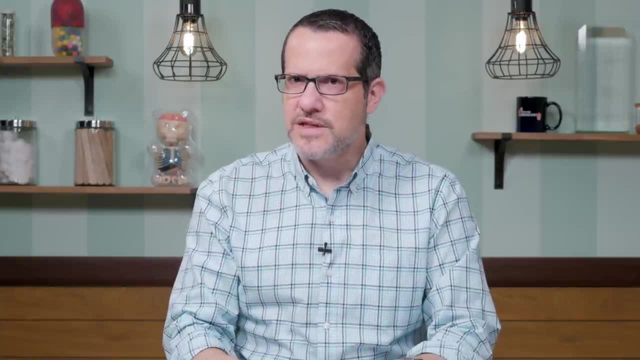 However, years before that evidence was available, some regions had adopted back surgery at a high rate, while others had not. Back operations performed in hospitals began to flatten after 2006,, but little was known about growth in the treatment in outpatient clinics, the same-day facilities with greater convenience. 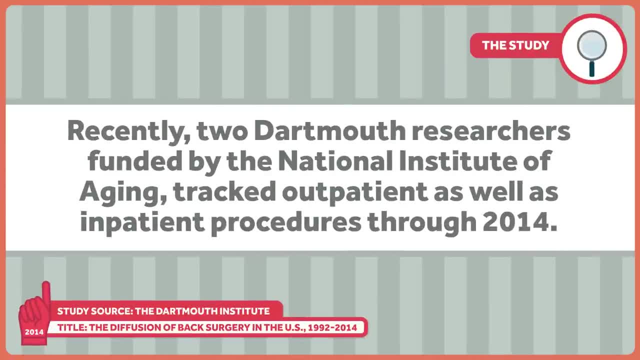 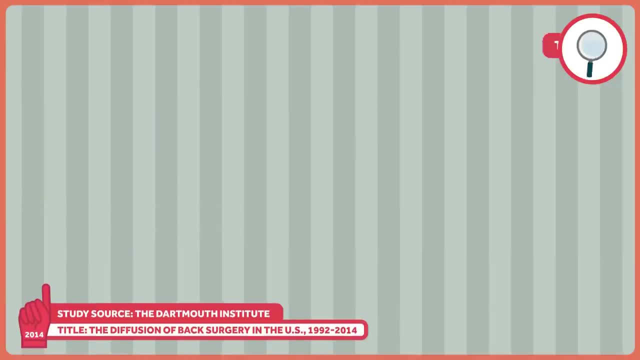 and lower costs. Recently, two Dartmouth researchers funded by the National Institute of Health and Human Services and the National Institute of Health and Human Services and the National Institute of Aging tracked outpatient as well as inpatient procedures through 2014.. Their finding Rates of Medicare back surgery had grown 28% since 2006,, with no 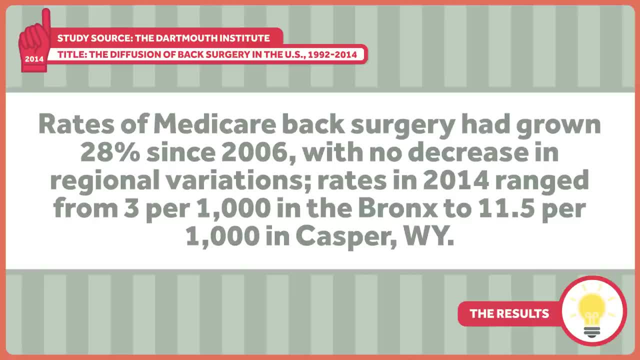 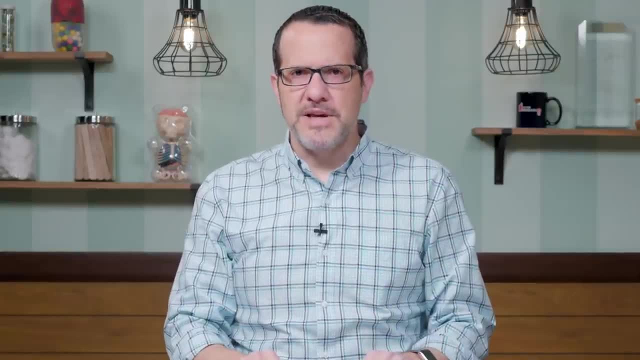 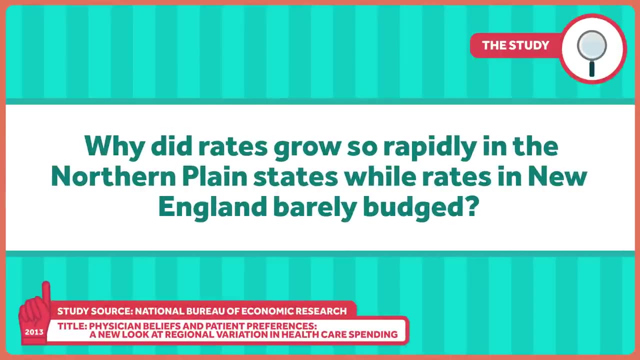 decrease in regional variations. Rates in 2014 ranged from 3 per thousand in the Bronx to 11.5 per thousand in Casper, Wyoming. The puzzling thing is why back surgery became more popular in certain broad regions but not so in others. Why, for example, did rates grow so rapidly in the 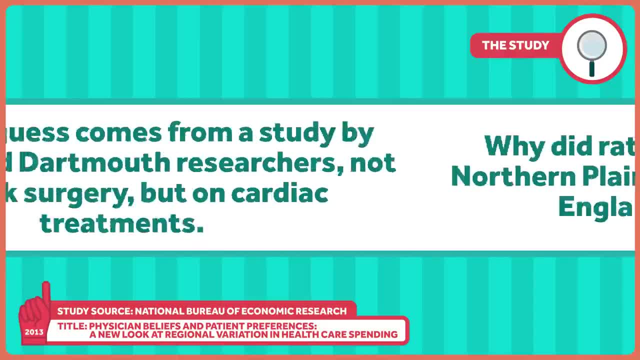 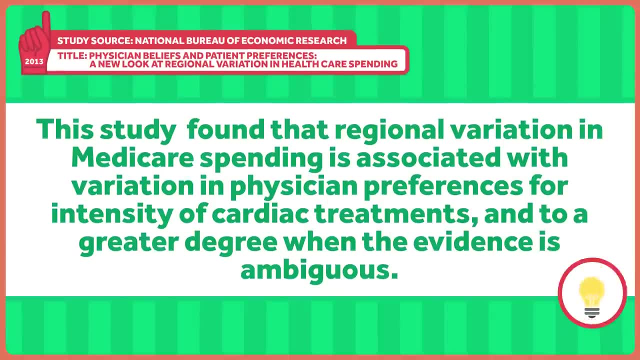 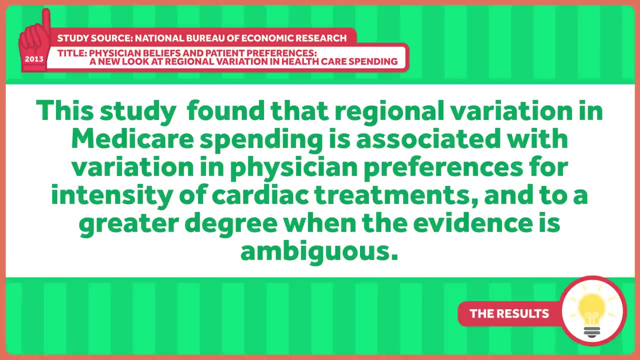 northern plains states, while rates in New England barely budged. Our best guess comes from a study by Harvard and Dartmouth researchers, not on back surgery but on cardiac treatments. It found that regional variation in Medicare spending is associated with variation in physician preferences for intensity of cardiac treatments. 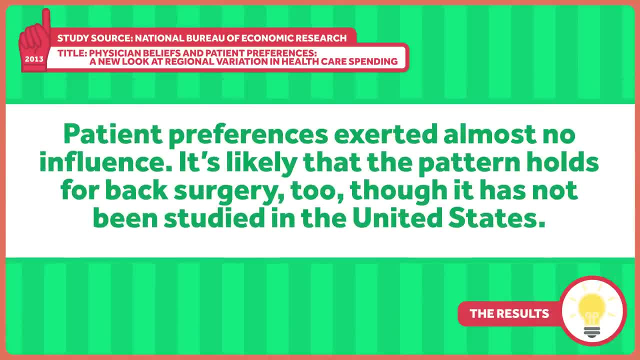 and to a greater degree when the evidence is ambiguous. Patient preferences exerted almost no influence. It's likely that the pattern holds for back surgery too, though it's not been studied in the United States. It's tempting to conclude that there are simply regions where the intensity of care of all types is higher that some regions invest in all of the latest shiny technologies while others don't. That's too simple. Miami, Florida and McAllen, Texas, the two most expensive regions in the United States for overall Medicare spending, also clock in with among the lowest spine surgery rates. Instead we see what Mr Winberg calls a surgical signature. Casper Wyoming has the highest back surgery rate in the country, but its cardiac bypass surgery is well below the national average. This puzzling pattern once again points to idiosyncratic physician beliefs Orthopedic. 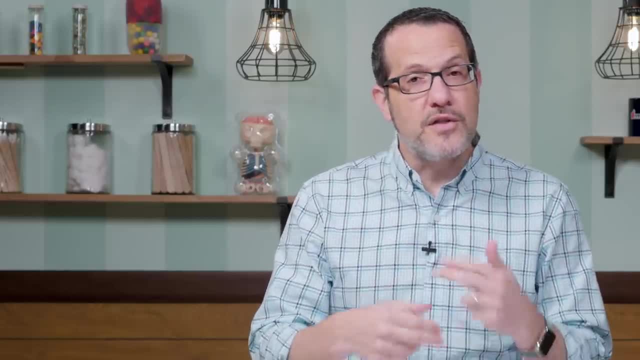 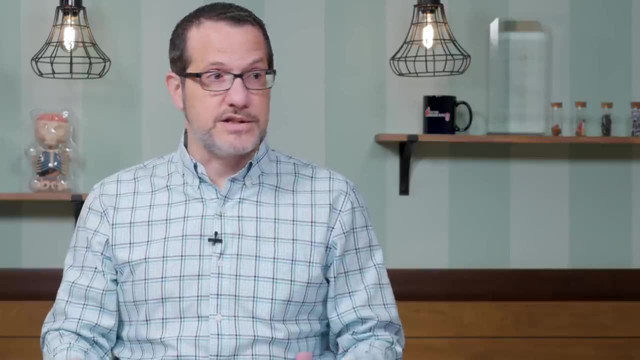 surgeons in a particular hospital may be more aggressive, while the cardiologists there are less so. Though we can't say this is the answer with 100 percent certainty, we can rule out some other explanations. One is how much surgeons are paid, Since Medicare pays. 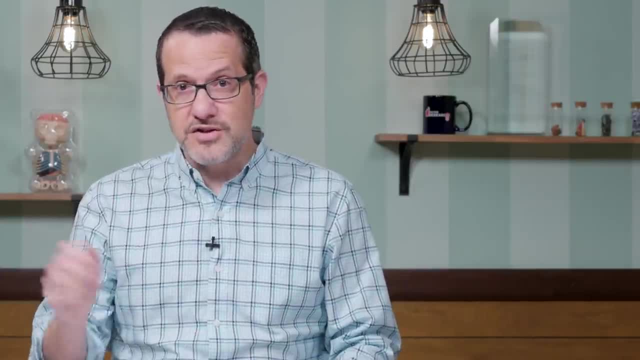 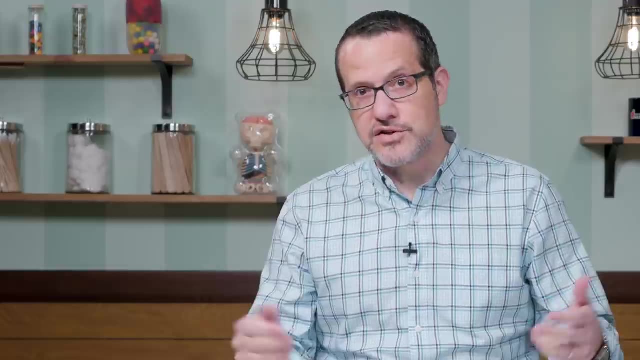 the same price for the procedure adjusted for cost of living across the country. prices can't be measured. The higher rates in Denver could also be explained by back pain sufferers who flock to star surgeons in well-known hospitals there. but that doesn't hold water either. The way the 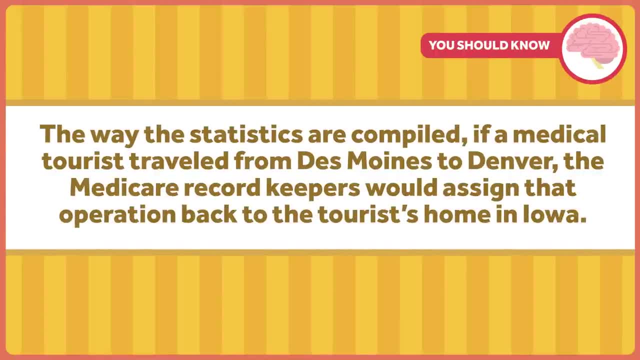 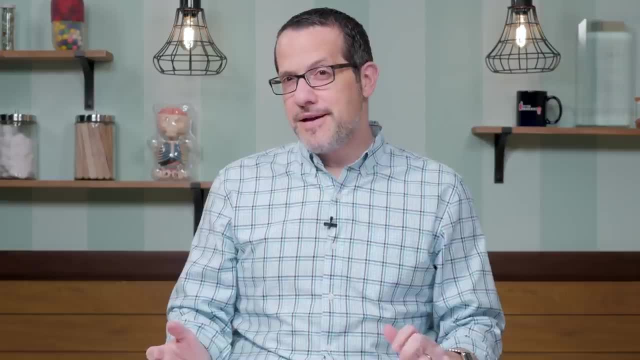 statistics are compiled. if a medical tourist traveled from Des Moines to Denver, the Medicare record keepers would assign that operation back to the tourist home in Iowa. Maybe it's differences in health? Perhaps areas with rapid growth in back surgery were those where more people had back pain. 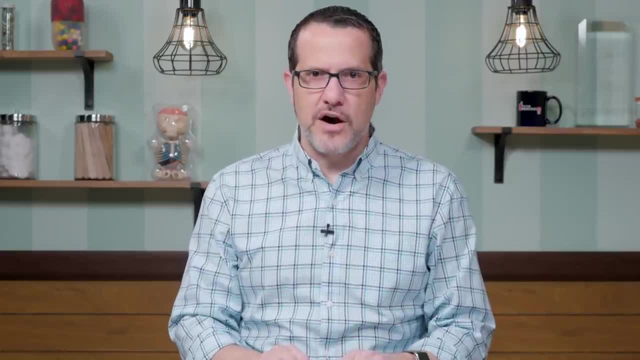 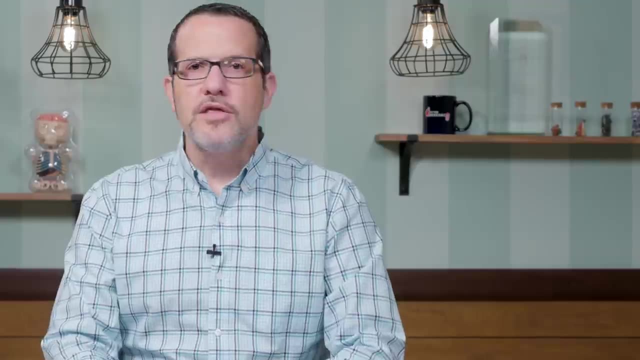 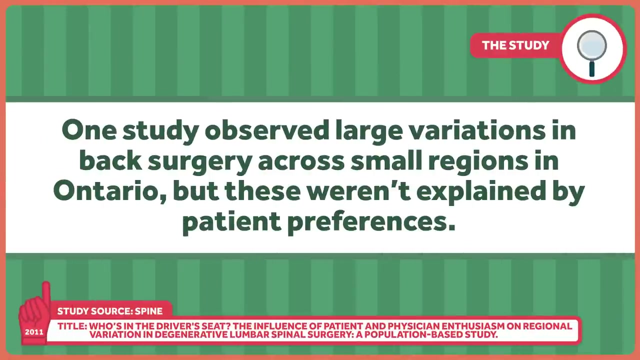 yet northern New England retirees had similar histories of hard physical labor and farming, lumbering and manufacturing, and were no more affluent than their counterparts in the northern plains states. Another explanation might be that patients prefer surgery in some regions of the country. One study observed large variations in back surgery across small regions in Ontario.